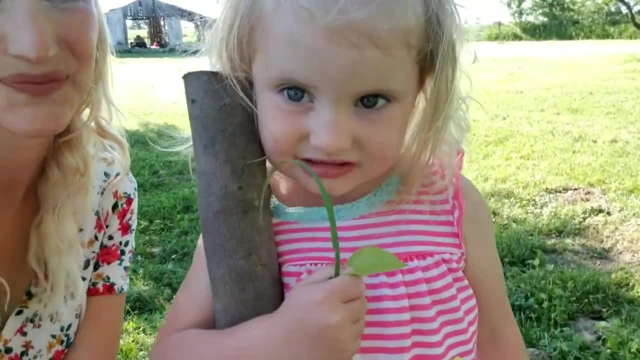 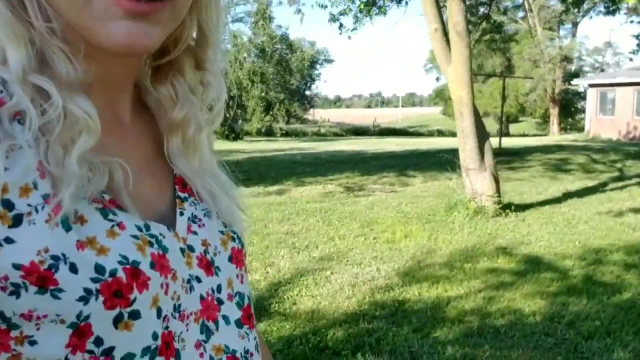 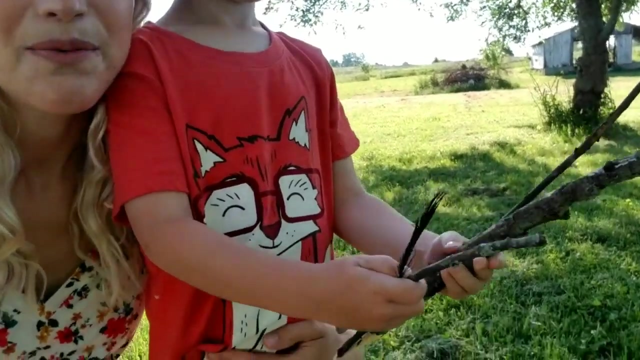 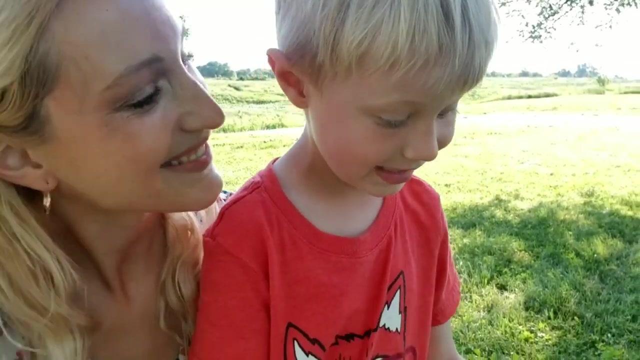 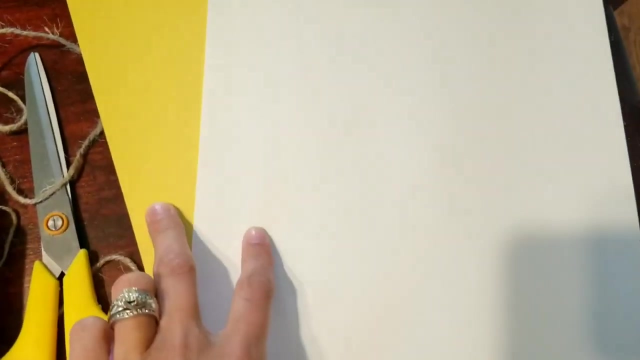 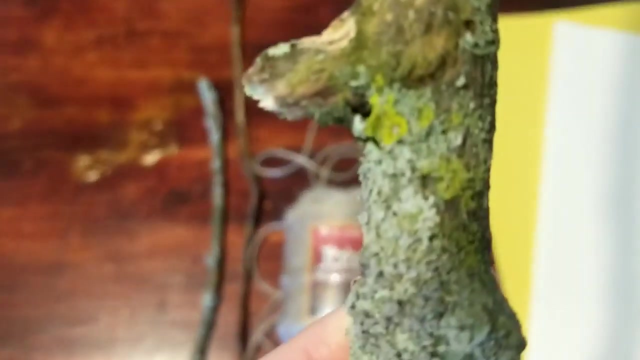 You found a leaf, some grass and big sticks. You found a leaf, some grass and big sticks. Good job, Hey Oliver. come show Mommy your sticks that you've got, you got, I got this. Show Mommy, Let's go get some more wreaths. Wow, Three, Mr Fox. Only I have three sticks. Let's go find more. Alright, so for our creation mobile, all we need is some paper for the sun and the stars, some scissors for the time and some sticks that we just found this morning from our nature walk. 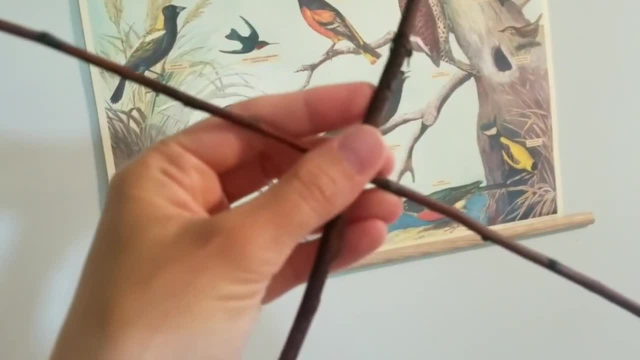 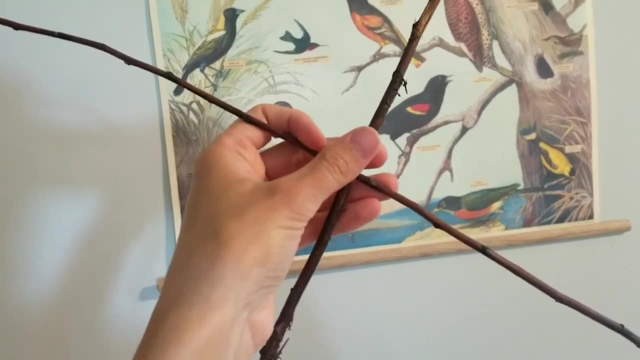 So all we have to do is we have to put some twine on the middle part here, see, And that will hold the two sticks together. Then we can put our fourth day of creation on it And we have our twine on in the middle, holding it together. 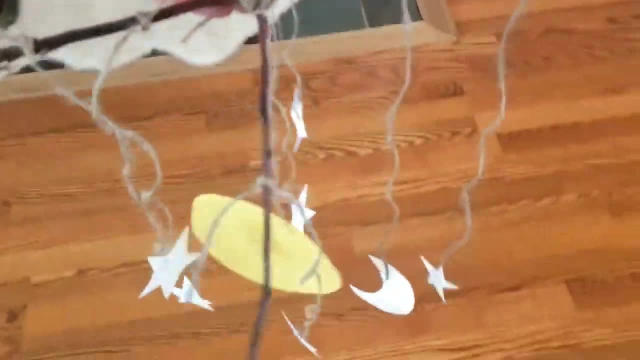 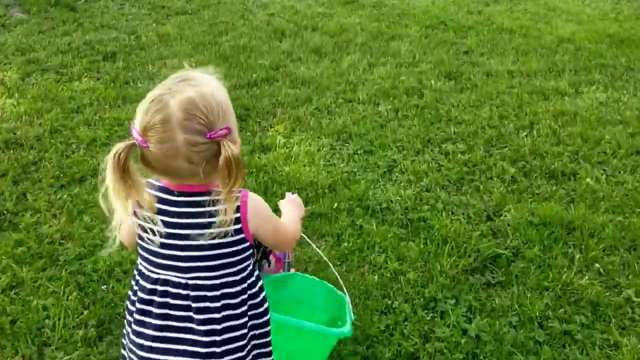 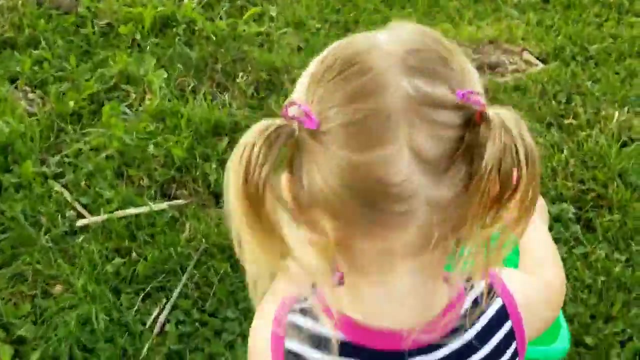 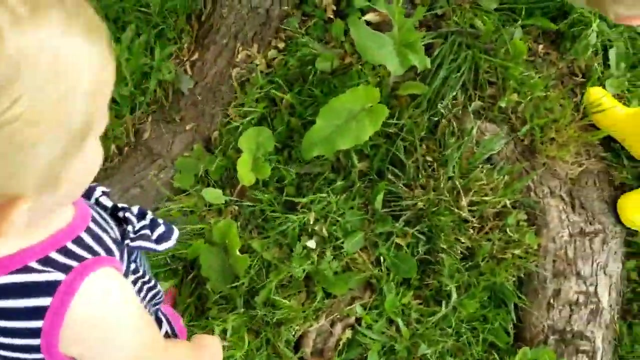 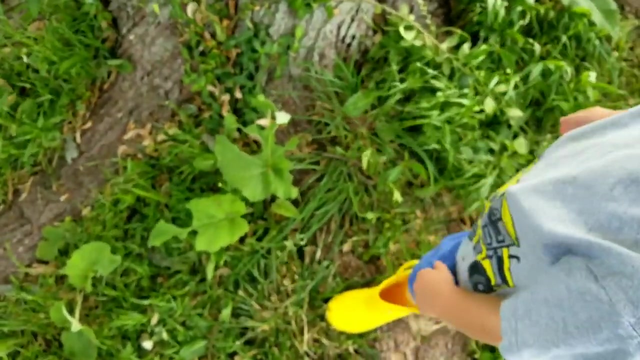 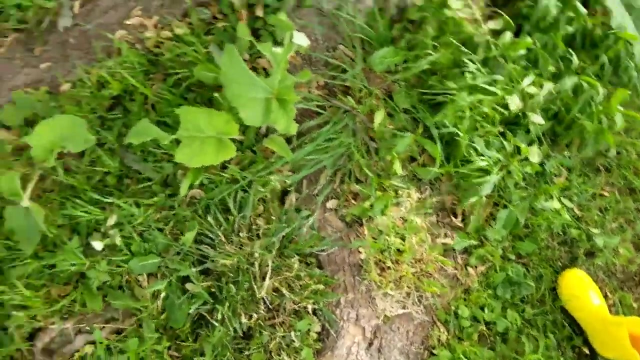 So today we started week five of our curriculum and this week's study is all about leaves. We're going to pick some leaves For this particular activity. they were searching for a bunch of leaves to dry out and use them for counting. later We're going to have to see what we can find. 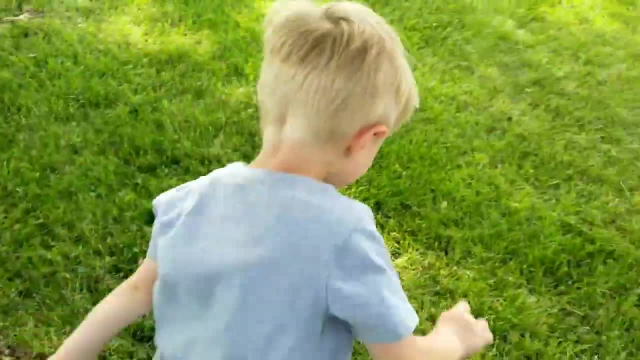 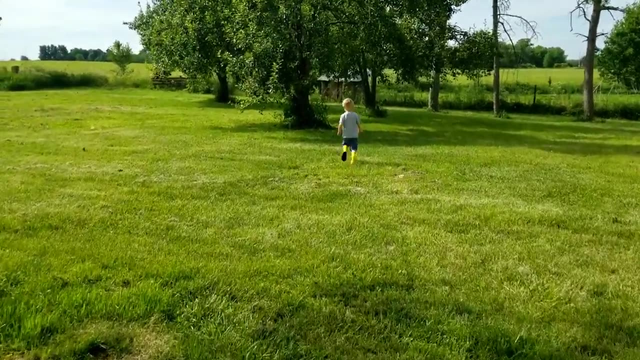 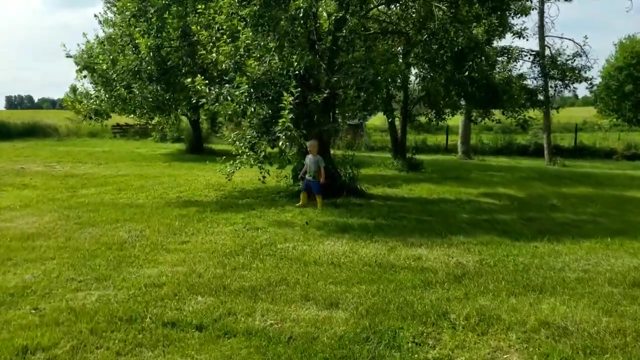 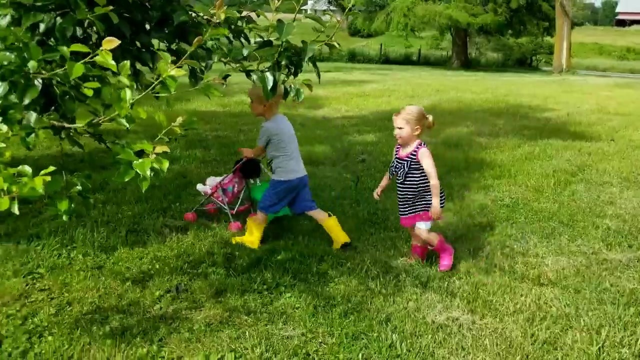 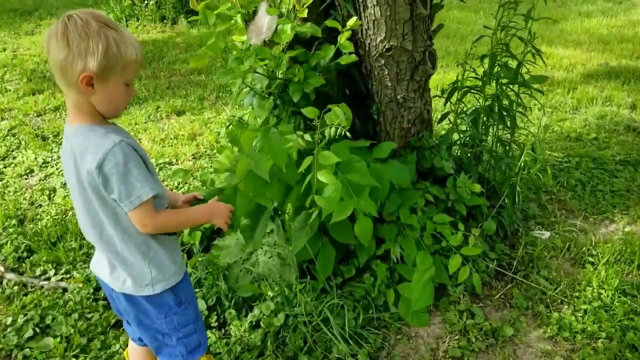 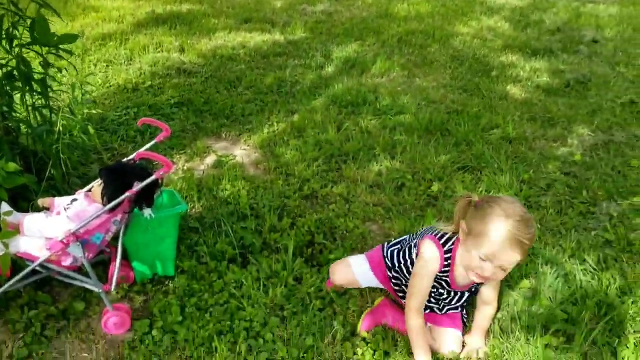 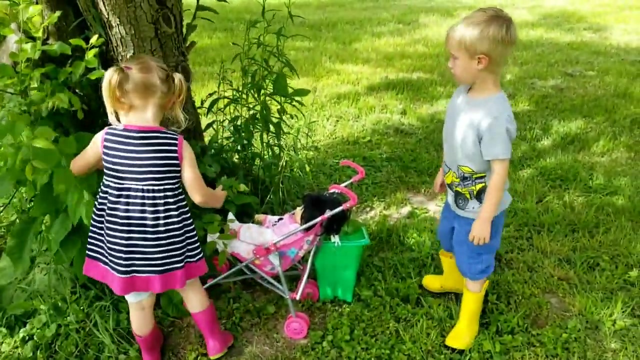 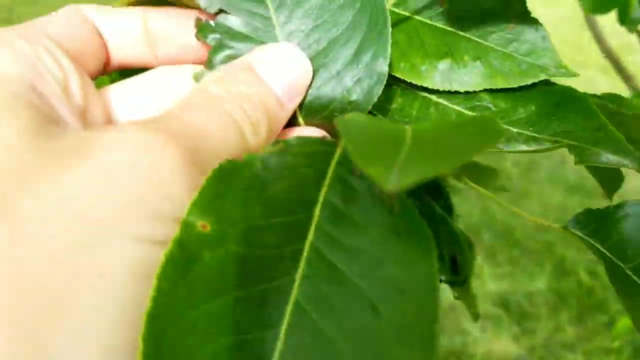 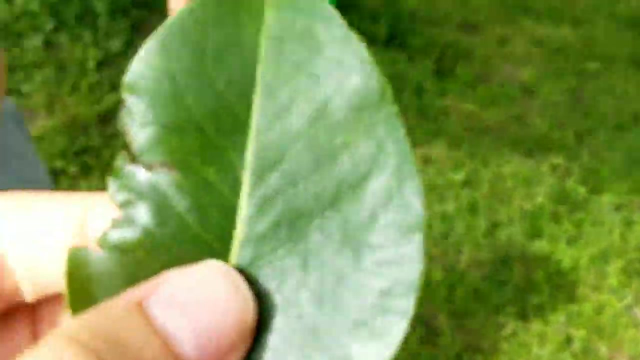 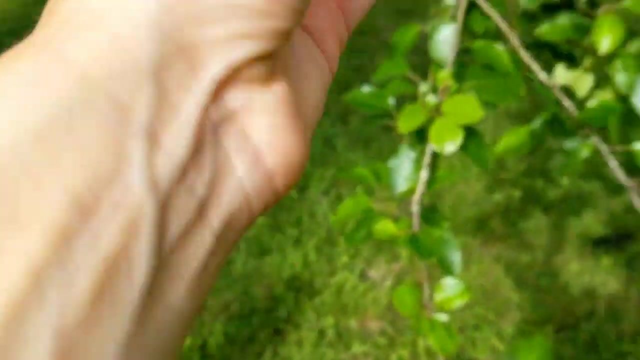 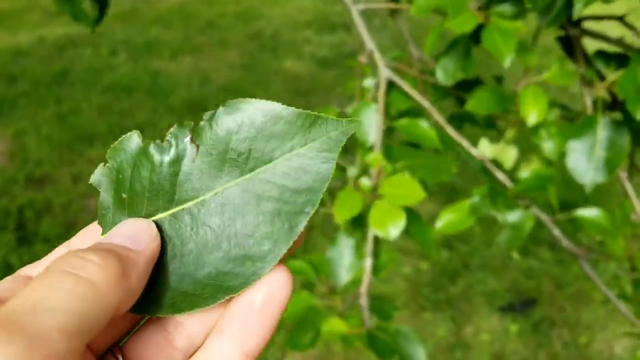 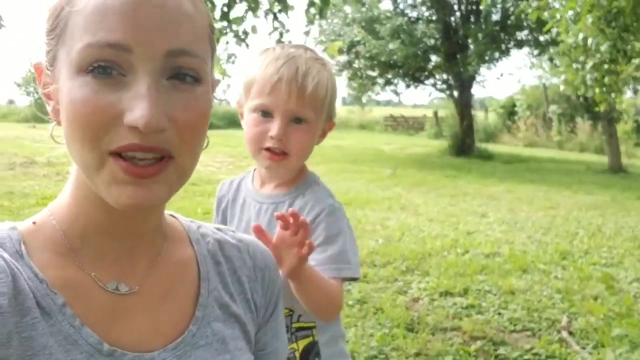 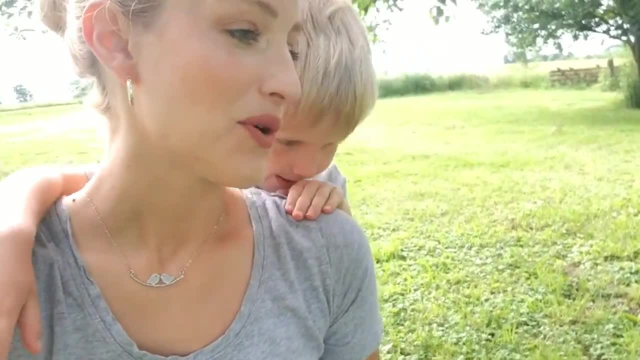 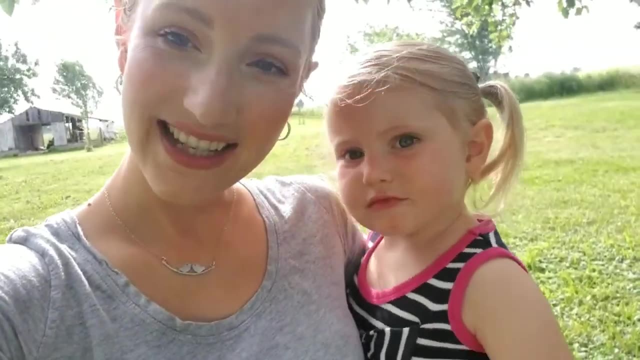 We're collecting leaves. We are collecting leaves, We're going to put them in a book and we're going to dry them out. Can you say hi to everybody? Say hi, Say hi, Say hi. No, we got a shy one. 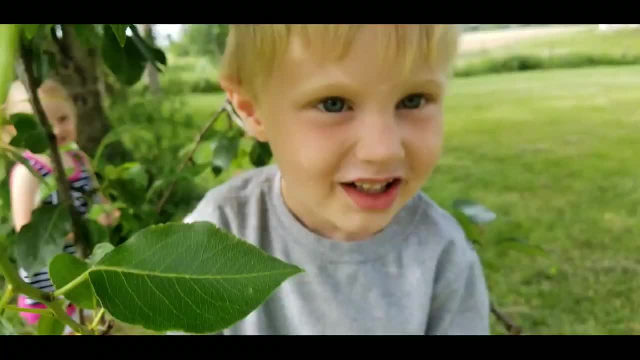 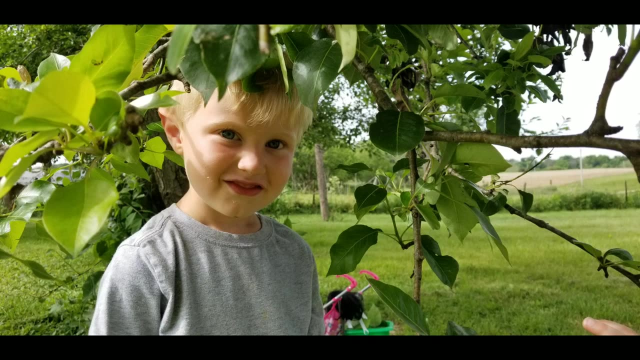 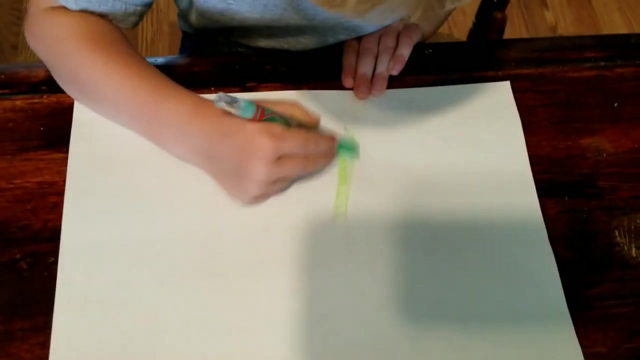 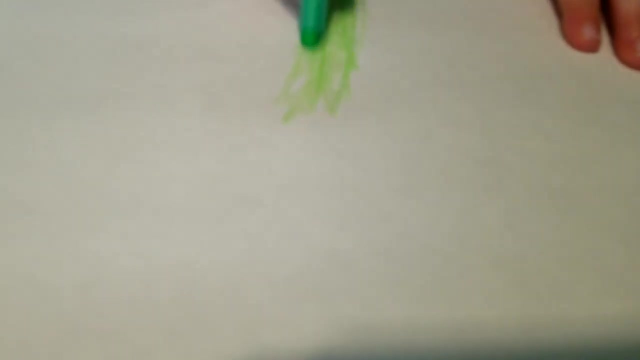 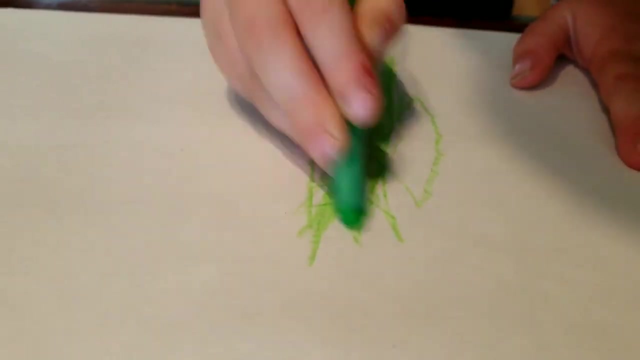 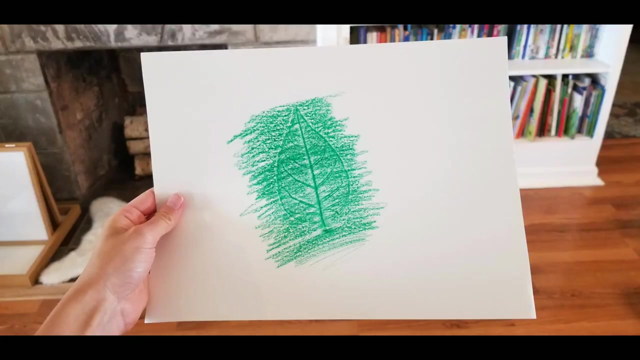 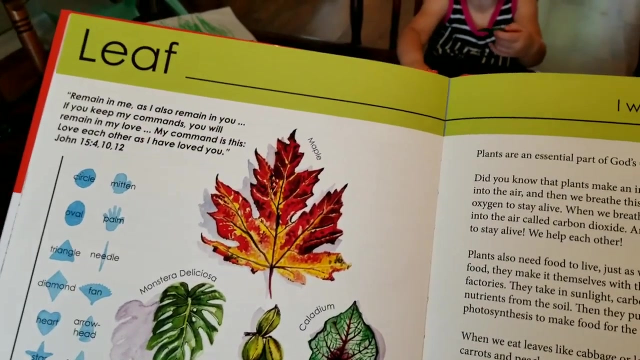 I see you, We're doing some leaf rubbing. See the veins starting to appear. They're starting to appear. Look at that. If you color it sideways, you'll also get them to appear as well. While the kids were finishing their leaf rubbing, I went ahead and did their reading assignment for today. 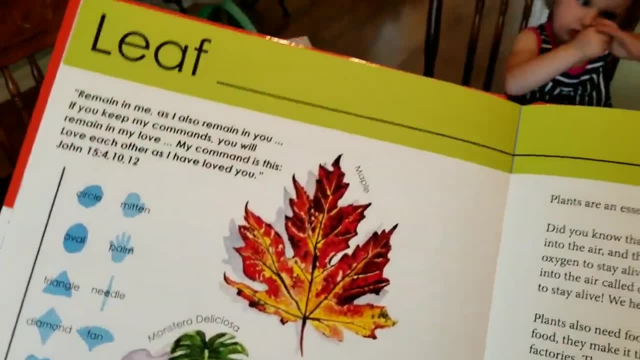 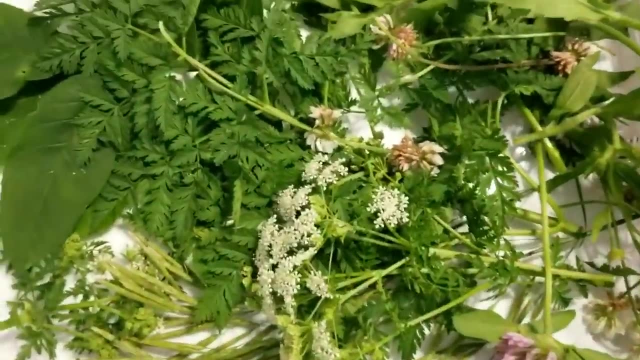 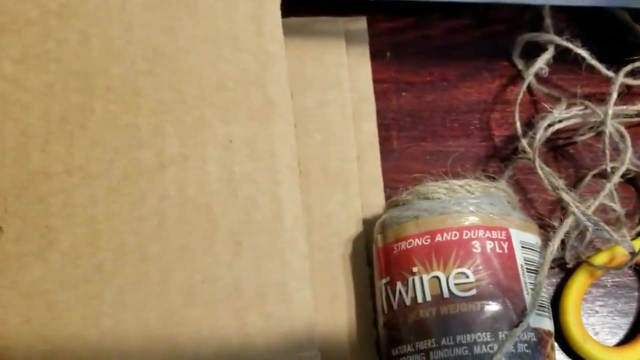 which was out of the book God's Amazing World. It's a great way to introduce both the Bible and science together. So for our last nature craft of the day, we decided to do little nature journals. We just cut apart some five by seven sheets of cardboard. 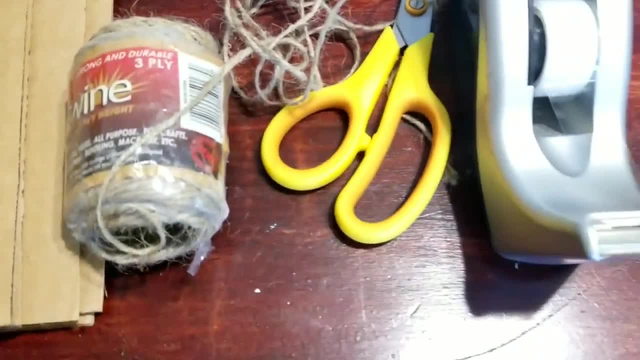 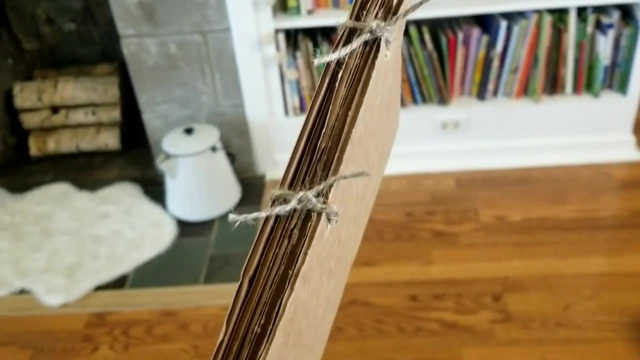 You can use any cardboard box And then just using twine, again with your scissors and tape, and that's it, and it turned out really durable. The kids are excited to take all their little nature clippings and findings and create some beautiful pages in their new nature journals.